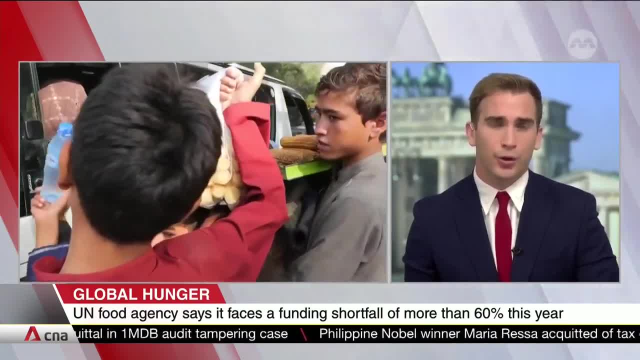 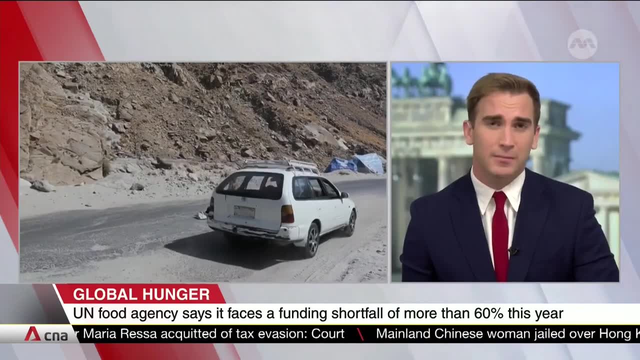 hotspots that they are seeing this situation particularly bad include Bangladesh, Afghanistan, Haiti and Syria. In fact, in Afghanistan alone, they've had to cut their budget by some 60 percent, And for that reason, they are saying today that governments do just need to do more to. 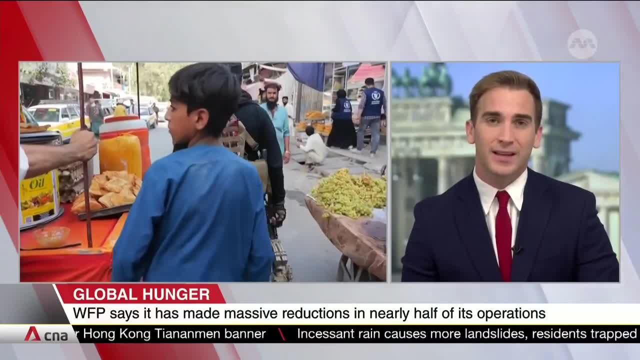 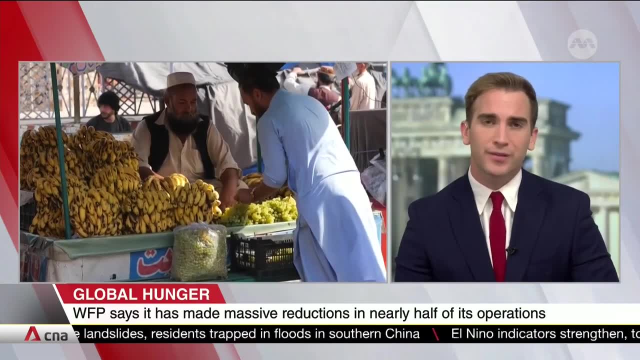 try and help them, They say. for the first time in their history, in fact, they are seeing a massive jump in their services being required, And yet their budget is shrinking. One of the other major issues they say they are facing is the shortage of food and food supplies itself. 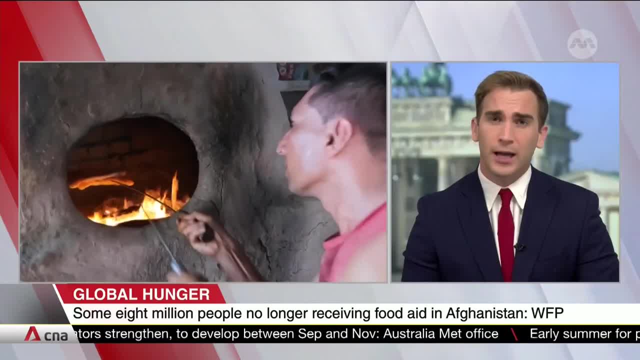 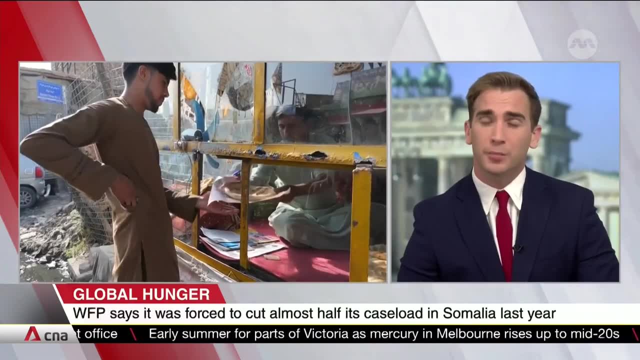 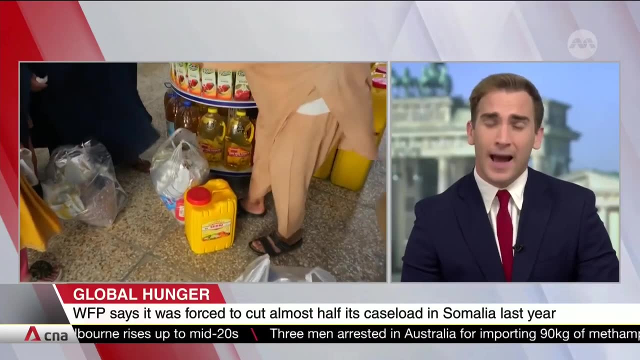 particularly because of that Ukrainian grain deal collapsing. We know Ukraine is often being described as the breadbasket for some parts of the world and the fact that grain exports there have dropped significantly because of the war that is having a major impact on those that are most vulnerable, particularly in Africa and also. 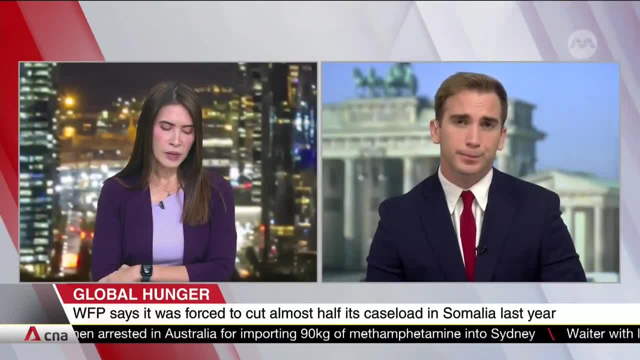 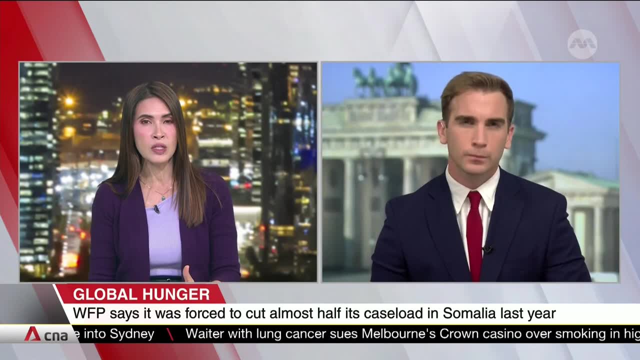 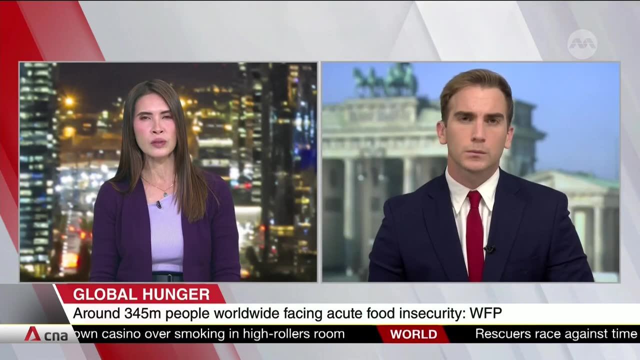 parts of the Middle East, Trent. the fact is that global needs are rising here and the World Food Programme, I mean, as you've just said, it wants governments to do more, but government contributions are on the decline. What are the reasons for this shortfall? 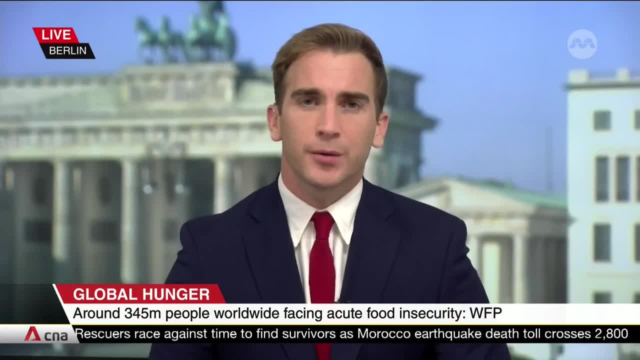 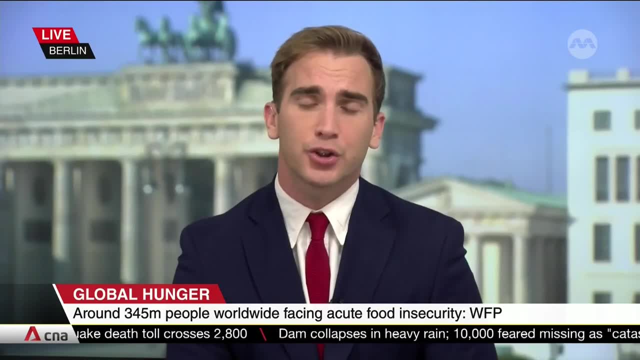 Well, I think the reality is that for many political systems, we see debates and discussions around budget shortfalls And, of course, we know that foreign aid budgets are just so often the first thing to be cut, given the economic uncertainty which has impacted certainly the 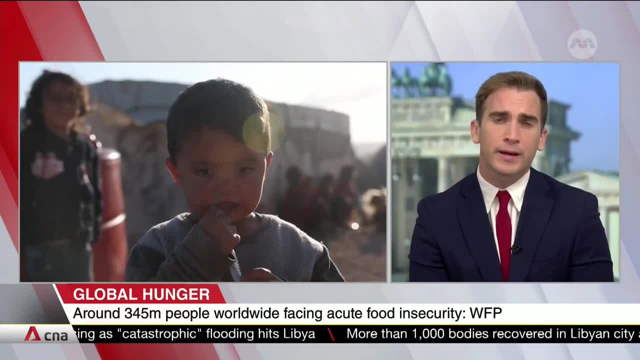 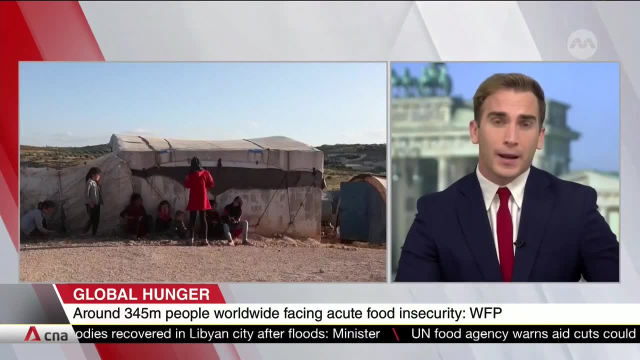 European Union, where I am, but also, of course, the US to some degree, with record inflation. We just know that our budgets are tightening, at a governmental level, but also at a personal level. Households in many cases have got less. 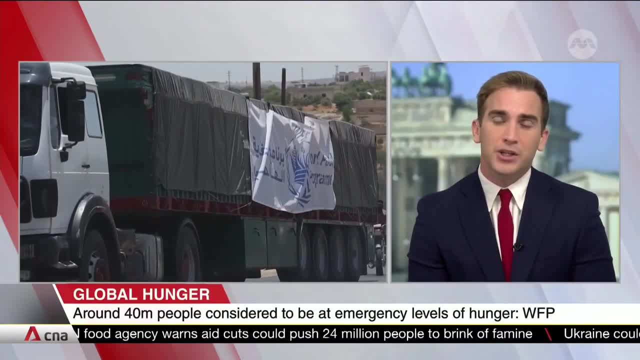 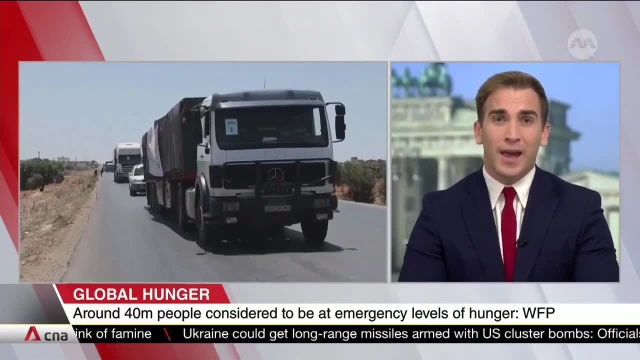 money to spend, less disposable income because of inflation, And that means that there are just less private donations going in as well. But, as I say, the World Food Programme is saying that those economic problems that perhaps the West is feeling well, they are also being felt. 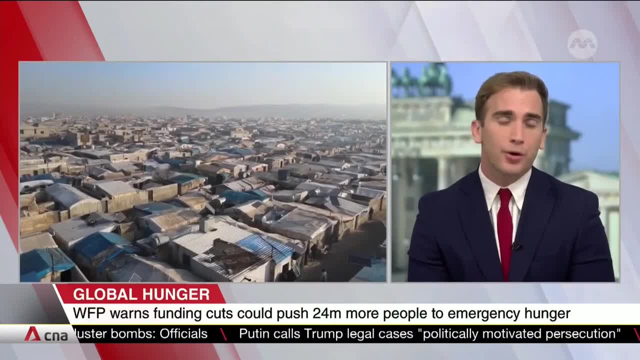 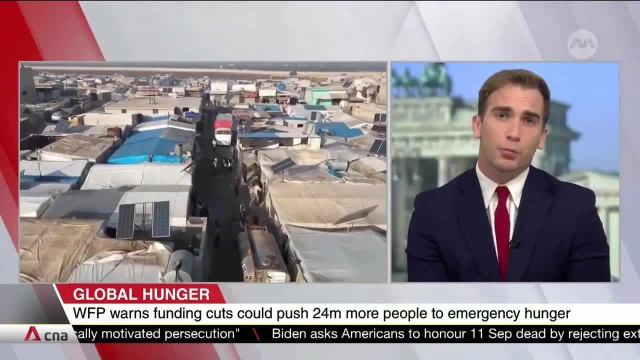 very much so in the developing world, And it is there that people are most vulnerable, And that is why, today, Cindy McCain, who leads the World Food Programme, is calling on both governments and citizens to do more to help them make up that double-digit budget shortfall dawn. 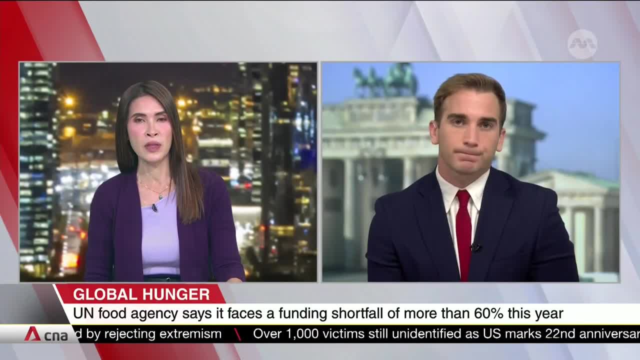 Some tough choices ahead, Trent. thank you very much for that. Trent Murray, there reporting live for us from Berlin.